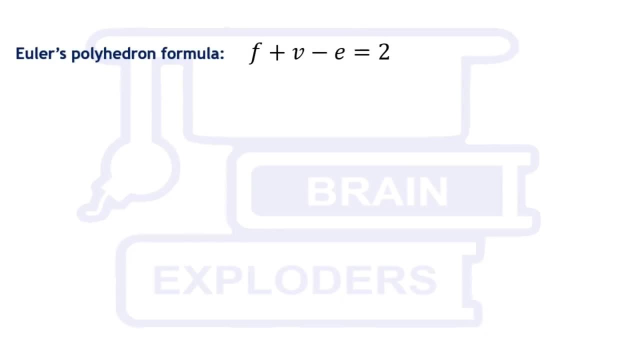 F plus V minus E equals to 2.. Let's see what this equation represents with the help of an example. Let us take a cube. We know that a cube has 6 faces, 8 vertices and 12 edges. So if we add 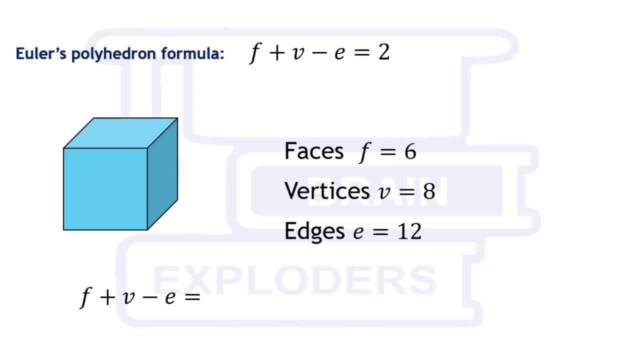 the number of faces with the number of vertices and subtract number of edges from it we get 2.. Is it true for all the 3D shapes? Let's check. Let's take this another shape. It has 4 faces, 4 vertices and 6 edges. So 4 plus 4 minus 6 is equal to 2.. It's a tetrahedron and this 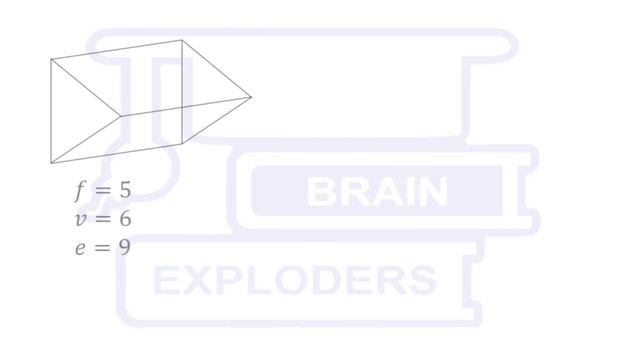 equation is true for this tetrahedron. also. Here let's check for the triangular prism, For this octahedron and for this square pyramid. So here, 5 plus 6 minus 9 is equal to 2. 8 plus. 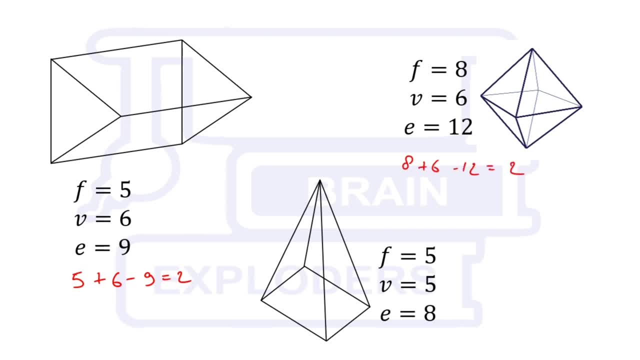 6 minus 12 is equal to 2, and 5 plus 5 minus 8 equals to 2.. This is Euler's polyhedron theorem, and it is true for all 3D shapes: that sum of the number of faces and vertices minus number of edges. 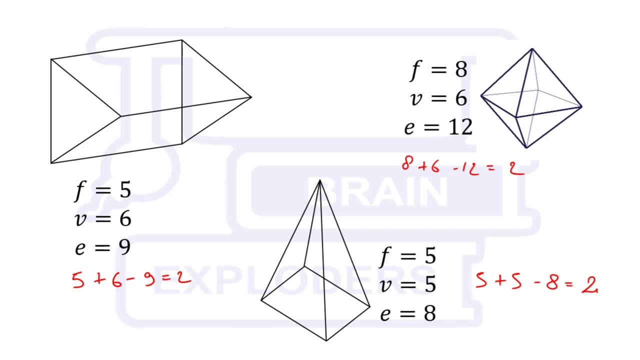 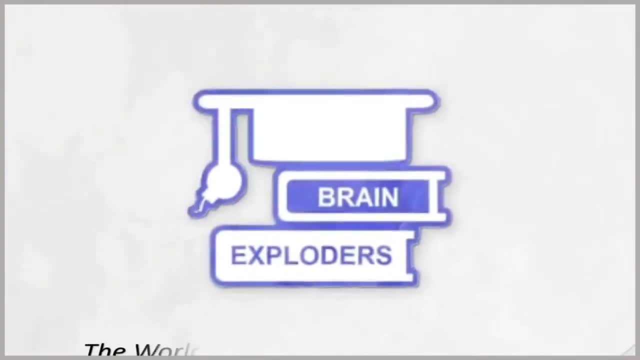 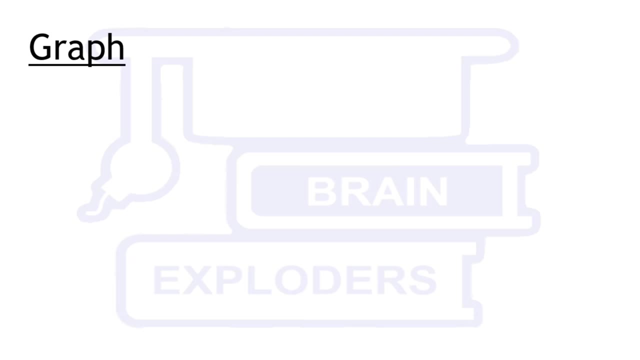 is equal to 2. And in this video we will see the proof of this equation. So, before going on the proof directly, we will discuss some basics of graph theory and what is graph. So we are not. we will not go in deep concepts of graph, We just 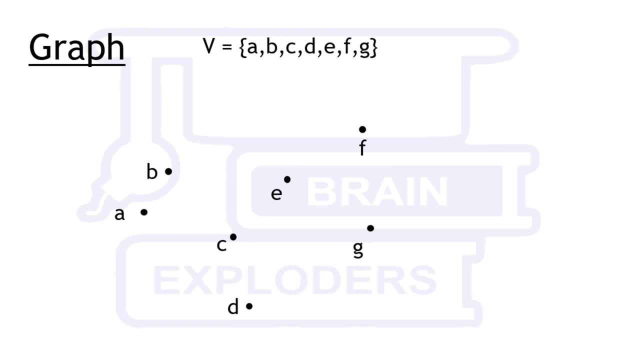 have to know that a graph consists of vertices and some connections between the vertices, which are called edges. Edges are the ordered pair. Edges means E set. E is the set of ordered pairs of elements of V. So that's enough for us to proceed. What is a planar graph, If any representation? 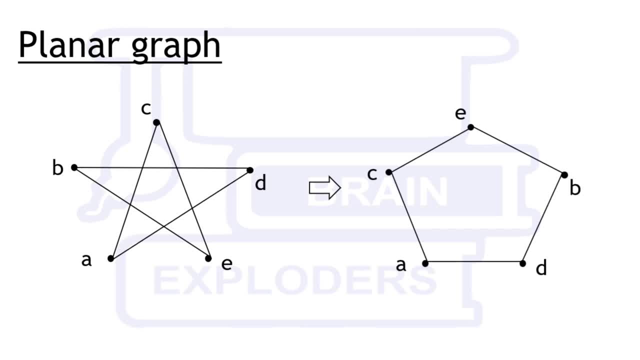 of a graph can be drawn in such a way that no edges intersect each other, then the graph is called planar graph. Here you can see that A is connected to D. In this graph also A is connected to D. A is connected to C here, So here also A is connected to C. In this way. all the connections in this. 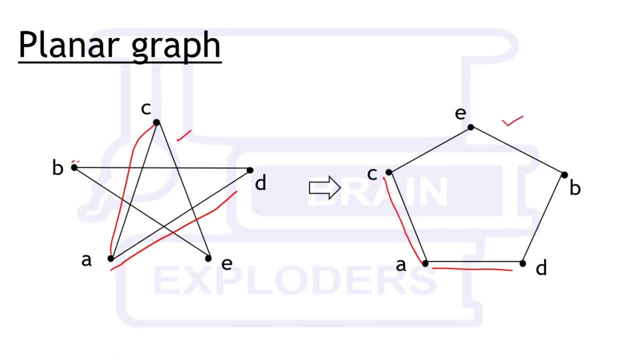 first graph is same as in the second graph, or we can say that both the graphs are same, and here this representation. in the second representation, no two edges are intersecting each other, as in this first one, and that's why this graph is called. this graph is a planar graph, but sometime, sometimes it's not possible for 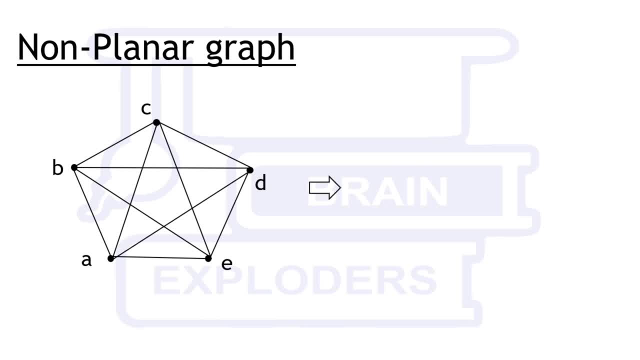 us to find any geometrical representation in which no two edges are intersecting means if in this graph, if you want to try to find some geometrical representation in which no two edge intersect each other, then you will not be able to find that. so, as you can see that I have tried to make 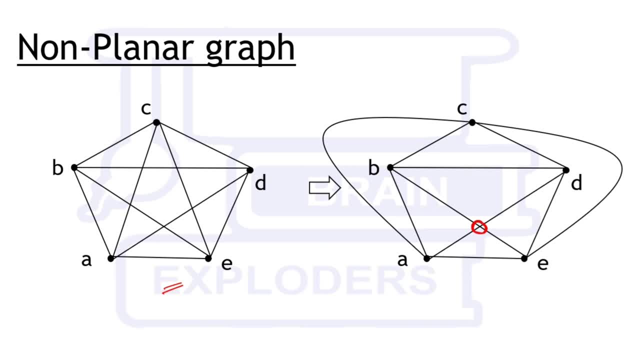 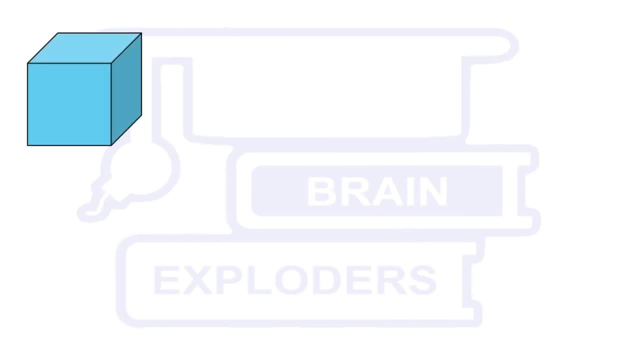 another representation, but here there is one intersection of edges, so it is a non-planar graph. so what we have to do, we will show some of the non-planar graph and we will show some of the non-planar graph and we will show some relation between some transformation, between the 3d shapes and planar graph. 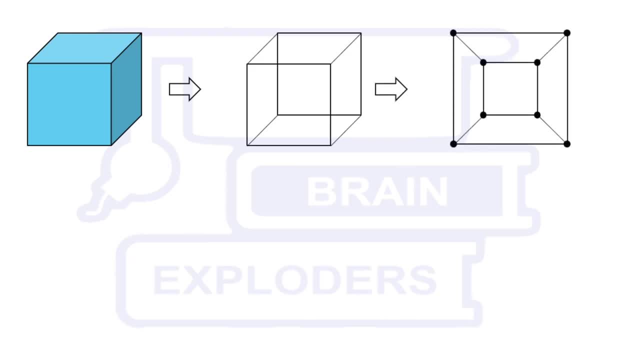 here you can see that this cube can be converted into a planar graph. can be transformed into a planar graph if we choose any one of the face of this cube. suppose this first face and stretch it. we stretch it means increase its size, so suppose you can assume that these surfaces are elastic and edges are. 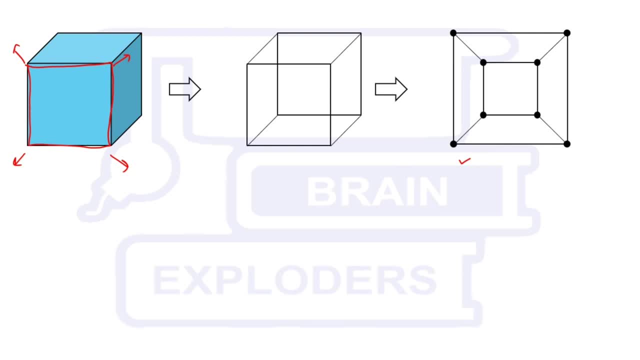 elastic and we can stretch them. so if we stretch this face and try to put all these vertices in a plane, then we will find this, this figure over here, here it has six faces, but here you can see that it has only one, two, three, four and five. 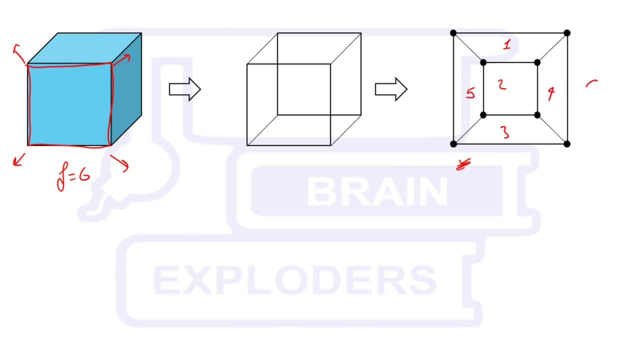 faces, so we will count this outer region also as one of the face. so in total six, or not only this shape, but other shapes or can also be- are transformed into other planar graphs. so suppose this are tetra, tetrahedral. add four faces: this first one, then here, the second one and the third one at the back. 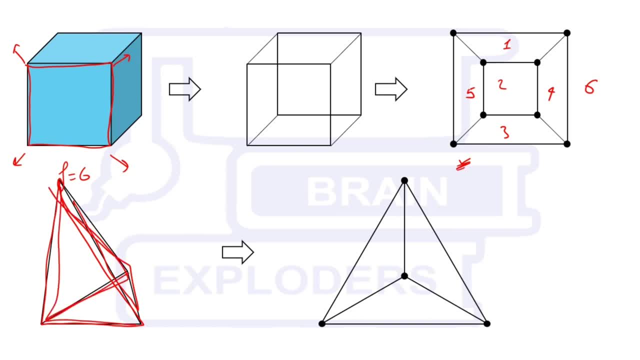 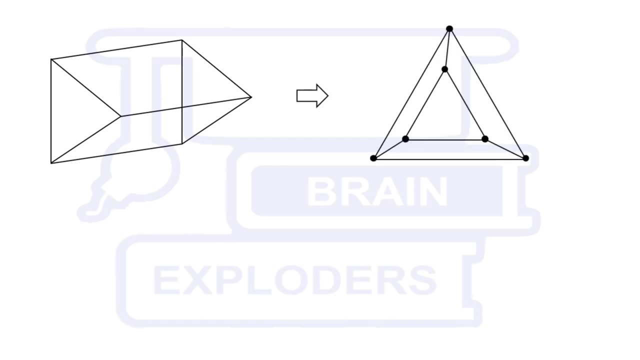 and this fourth one, at the bottom, this one. but this shape, this planar graph, only has three. so we will take this outer region as the fourth face. in the similar way, any of the 3d polyhedron, any of the polyhedron, can be converted into a. 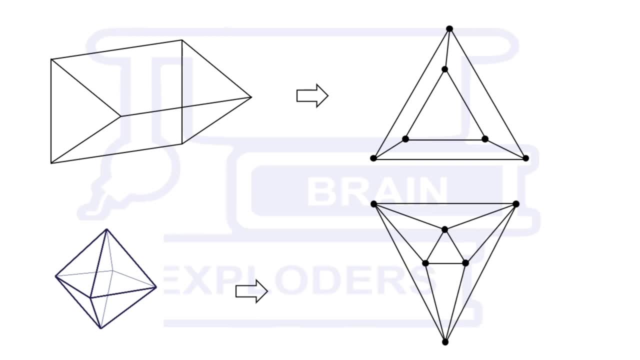 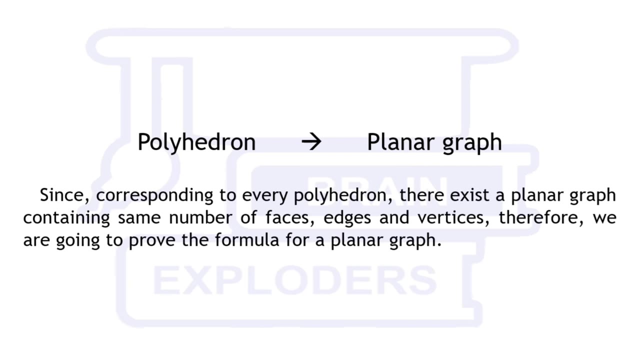 planar graph and since all the polyhedrons can be represented like the planar graph, as as we can see on the screen, so we will prove this theorem for planar graph and if we are, if we can prove this theorem from planar graph, we will. 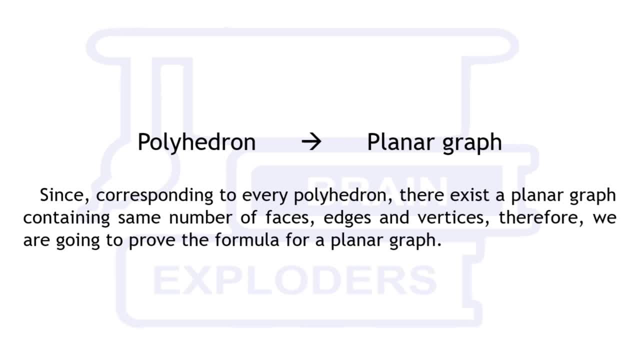 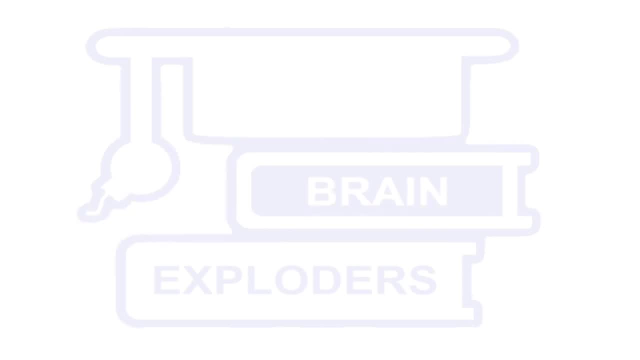 be sure that it's true for polyhedrons also, because all the polyhedrons can be converted into planar graph. okay, so let's start. some tools which we will use are here. some of the interior angles of a polygon is equal to n minus 2 pi, where 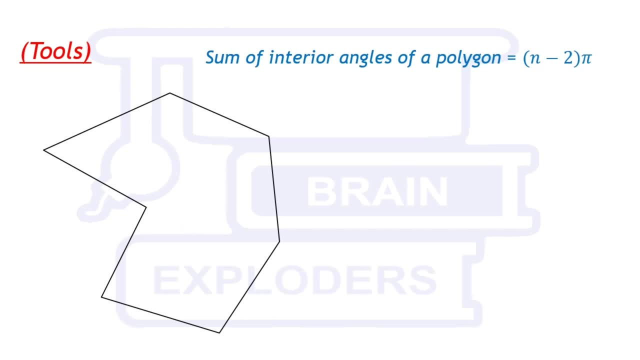 n is the number of faces that are in that position. then we can produce this pattern of sides of the polygon. So here some of these blue angles is equal to n minus 2 pi, and some of the outer angles means these angles which are shown by green color. actually I find terminology 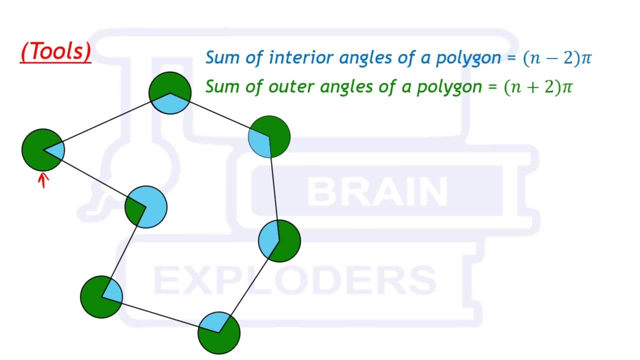 for this angle, but I didn't find the what is the name, what the name of this angle is, So I have written just outer angles over here. If some of you know what is the name of this angle, then please tell us in comments, because I know that it's not called exterior angle, So I have 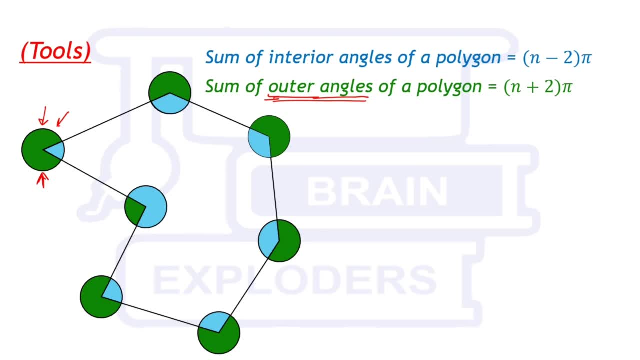 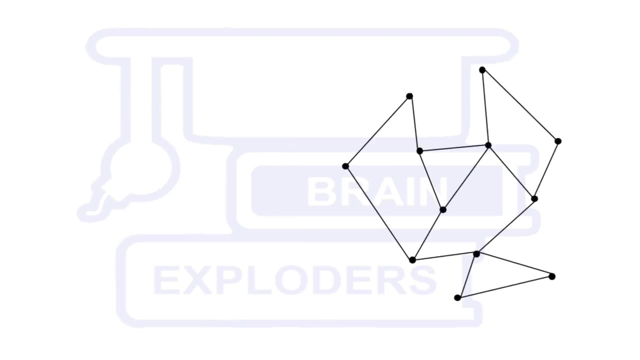 just using about outer angles. So sum of outer angles of a polygon is equal to n plus 2 pi. We will use these two results as tools in our proof. So let's start with this graph and let's analyze this with some very basic ideas. 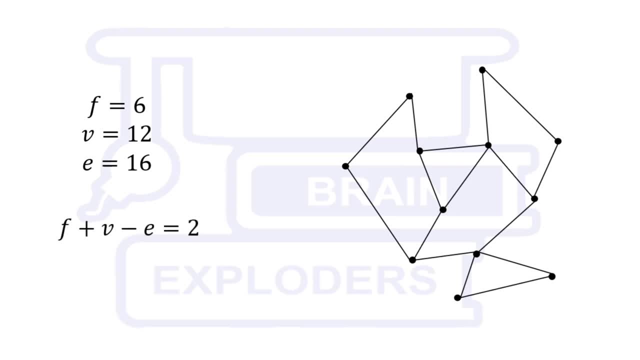 that why this equation is working. So here in this graph, including the outer region, it has a total of six faces here: 1,, 2,, 3,, 4, 5 and this outer one has 6.. It has a total 12 vertices and 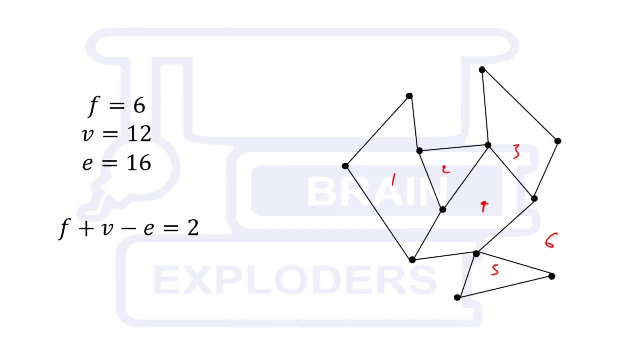 16 edges. So let's have a basic, a very basic idea that why this equation is working. So suppose, if we create another graph with the help of this graph and we increase an edge over here with the help of a new vertex, So here you can see that one vertex is increased. 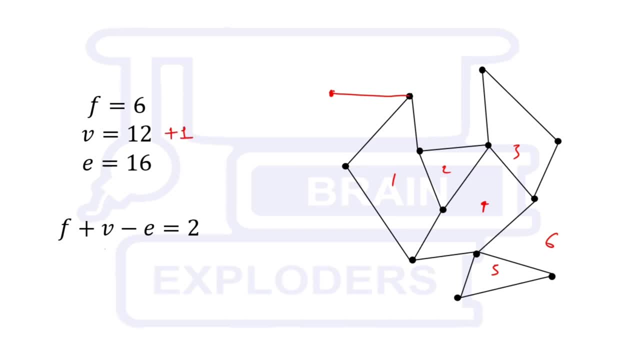 over here means now there are in total 13 vertices and one edge is increased. And in this equation, if we take this, f plus 12 plus 1 means 13 minus 17.. Thank you, So this is equal to 2.. Then it is also equal to 2. Since one is increased in this v and one is increased in this. 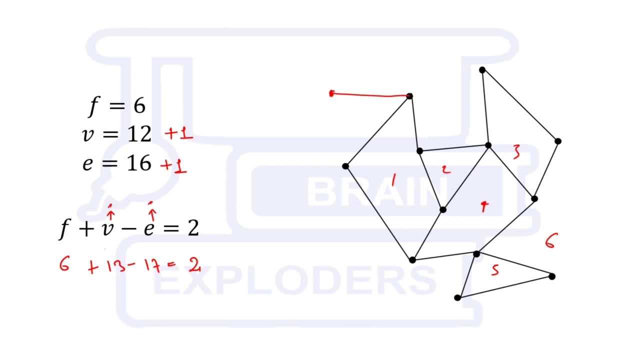 e. that's why it is they are maintaining each other means they are both increments are canceling out each other, and that's why this result 2 is maintained. But similarly, if we try to increase, or we, if you try to increase the edge by connecting any two vertices, suppose, sorry, yeah, any two vertices. 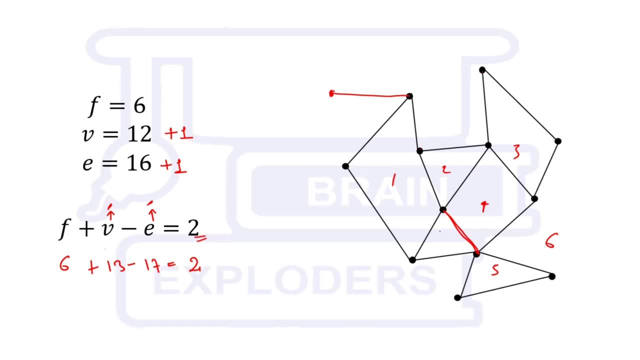 are made this edge over here. So here we have this seventh phase means there is an increment in the phase and an increment in the edge. So similarly, here also you can see that there is an increment in phase and there is an increment in edge and both these increments will cancel out. 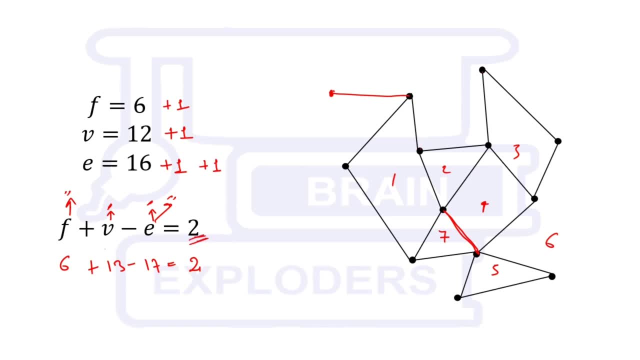 each other and the result will remain 2.. So if you want to calculate, then a total of seven phases here we have, and 13 edges, and, sorry, 13 vertices and 18 edges. So this result is still 2.. So it is the basic idea that how this formula is working. Now let's see a more. 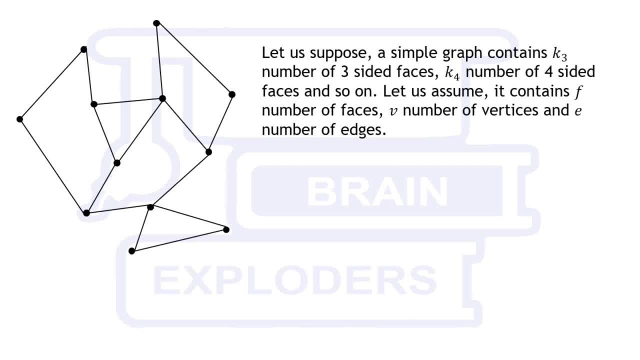 general proof. Let us suppose a simple graph means this graph like this, in which there is there are no parallel edges, something like this: no parallel edges and no loops. So we are talking about the graph, this, this type of graph. So a simple graph contains: k3- number of three-sided phases. k4- number. 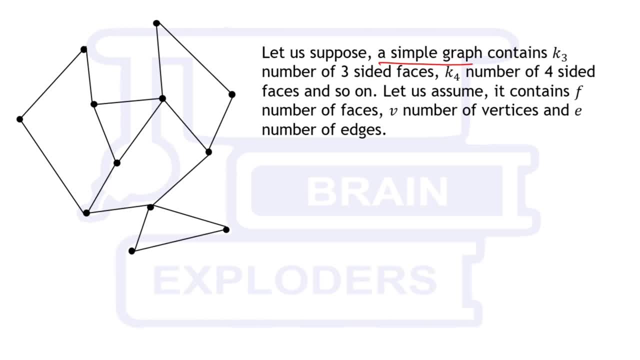 of four-sided phases and so on Means: let us here: this is the. this is a three-sided phase, this one and this one is a three-sided phase. So means k3 over here is equal to 2 and k4 is equal to 2.. So 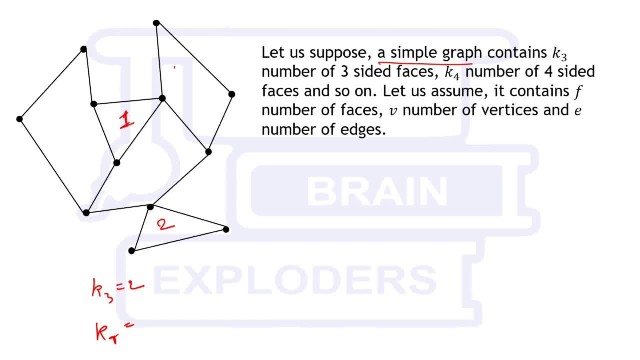 k3 over here is equal to number of four-sided phase, means 1, 2, 3, 4, this one and 1, 2, just one phase, So this one, k4.. Similarly, k5 means number of five-sided phases. So this is what: k1, sorry, k3,. 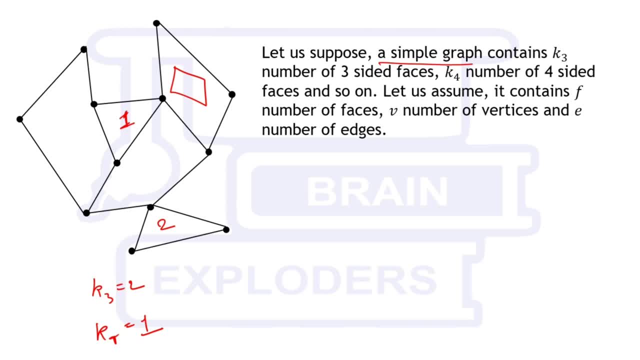 k4, k5, etc. represents. Let us assume it contains f phases, v number of vertices and e edges. So if we add, then k3 represent 3 number of vertices and e edges. So if we add, then k3 represent 3. 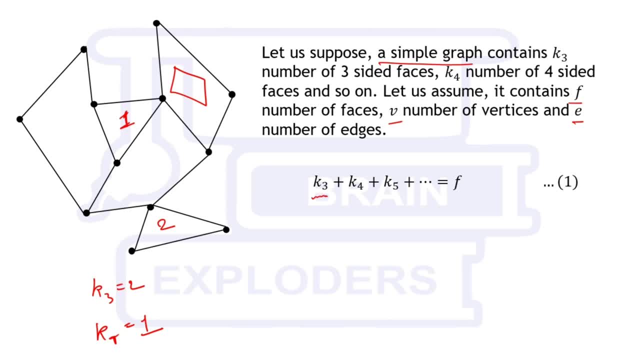 number of phases which have three edges. K4 represents the phases which have four edges, K5 represent four edges, so phases having five sides. So and we know that there is nothing like k2, because face cannot form by two edges, and there's nothing like k1, etc. So if we add this, k3, k4, k5. 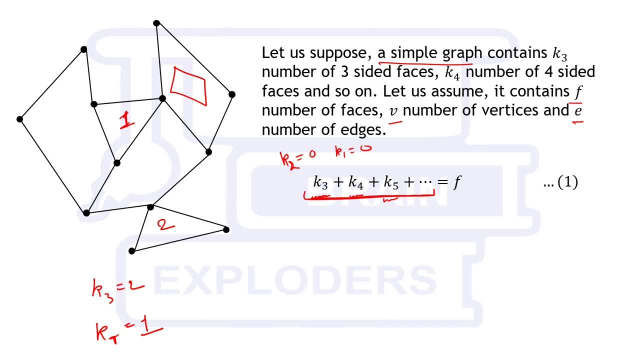 means we are adding the number of faces, and total number of faces are f. So here we get this first equation Now. 3k3 plus 4k4 plus 5k5, what is this? So 3k3 means this time we are trying. 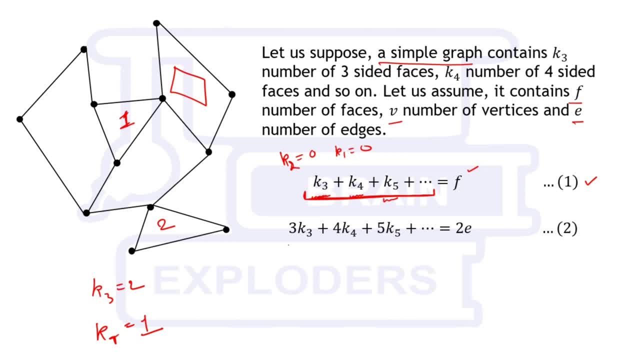 to count the number of edges. What is this? 3k3? Means number of faces having three sides is k3 and counting 1, counting 3, 4 each of such face means we are counting edges. So means 1,, 2, 3,. 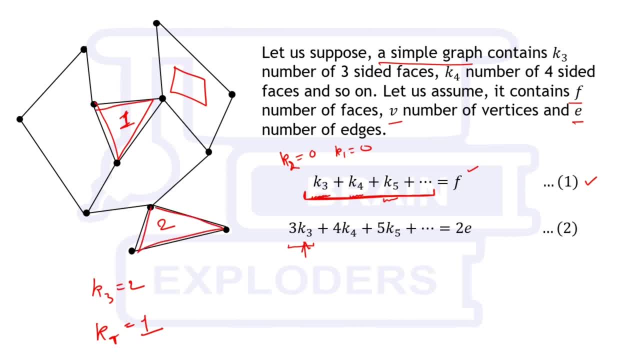 4, 5, 6.. So 3k3 means 3 into k3 means 2 into 3 means 6.. So that is why it is 6 over here Means this time we are counting number of edges. Similarly, 4k4 means this: 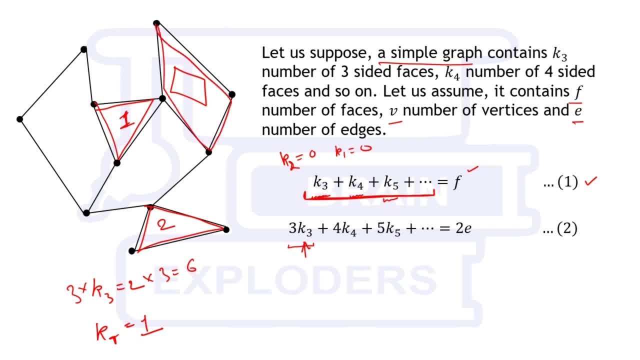 But you will notice that in this way, if we count the edges of all the faces over here, then we are going to count each of the edge twice. You can see that. if you can see that if I am trying to count all the faces, then edges of all the faces, then I am counting each of them as. 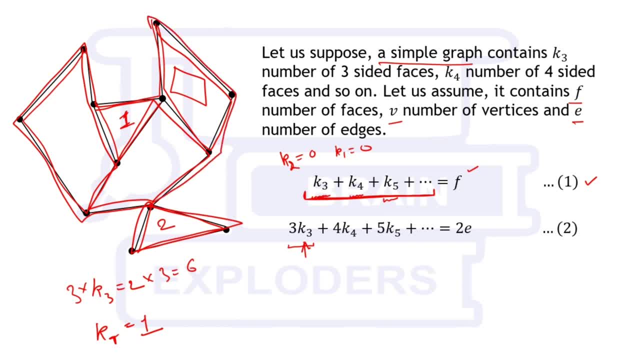 I am counting each of them twice. Look, and at last I have counted this outer region also. So since I have counted all the edges twice, that is why on the arches it is written: 2e means twice the number of edges. So 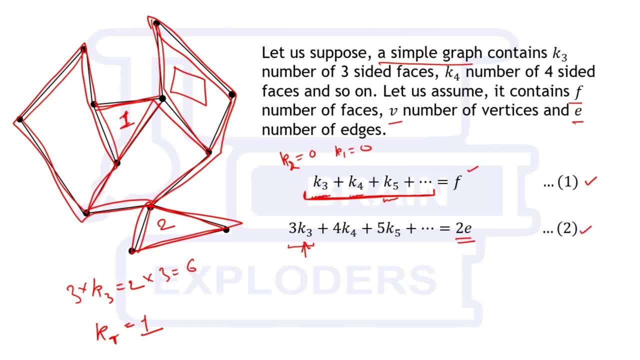 here we have the second result. We will use it in the proof. Sum of angles around the vertices is equal to 2vpi. I am talking about this angle, this overall angle around the vertices. It is pi. It is pi a solid. 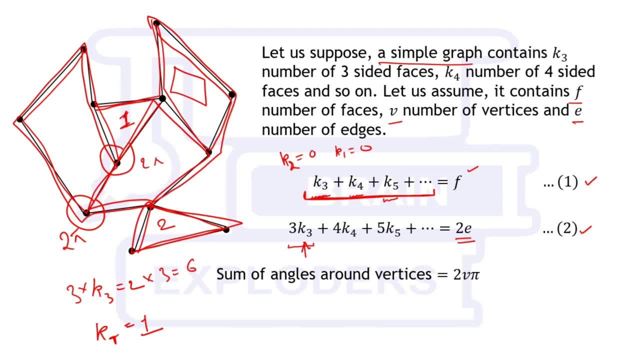 2pi. It is also here 2pi. This one is also 2pi. This one is also 2pi. So sum of all the angles surrounding the vertices is equal to 2vpi, because there are v number of vertices. This is our. 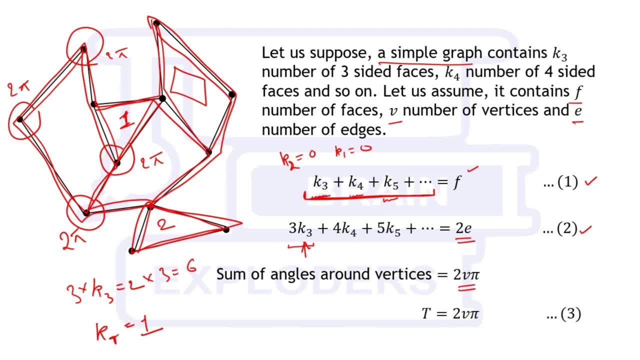 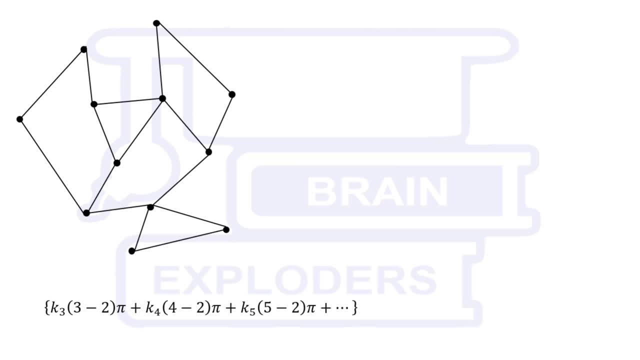 third result: Let us represent this sum as t. Now just look at this equation and later you will know that what you are going to Do? So k3 times 3 minus 2pi. I am using the formula for the sum of interior angles: 3 minus. 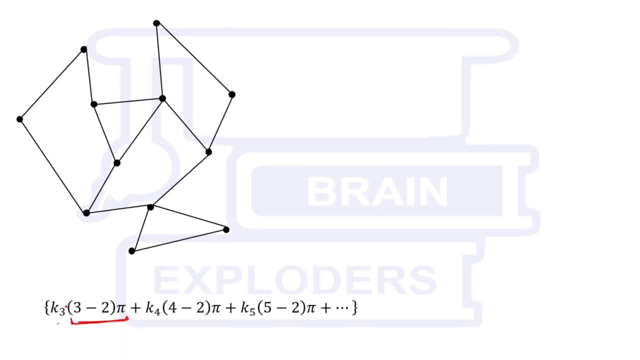 2pi- This represents the sum of interior angles of a triangle- means this one, And we are doing this for all the faces. having three sides means k3. number of times means this one also. Similarly here For k4, for k5, and here also 4, 5.. But one more thing here, since we are taking this outer region: 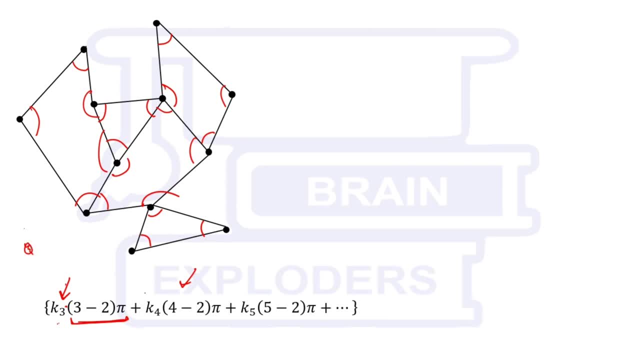 also. we are taking this outer region also. that is why In this equation there will be a face where we will count this. we will count the sum of interior angles of a face which is exterior like this. Sorry, not there Here, So we will. 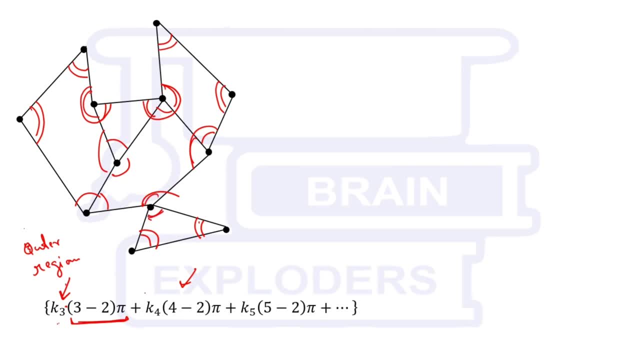 count, something like this. This also Okay Means for those vertices which are on the boundary, which are on the boundary we will. we are going to add this twice. Okay, We will wait for some time. we will know why we are doing this. So here this formula, or whatever this expression is. 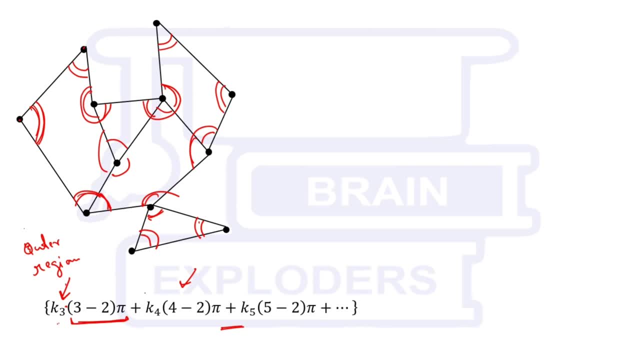 written will do something like this: Nice Now plus xkx means if we want to add this outer, we don't know, we don't know that how much number of sides this outer region is going to have. So we will add this x plus 2 times pi. 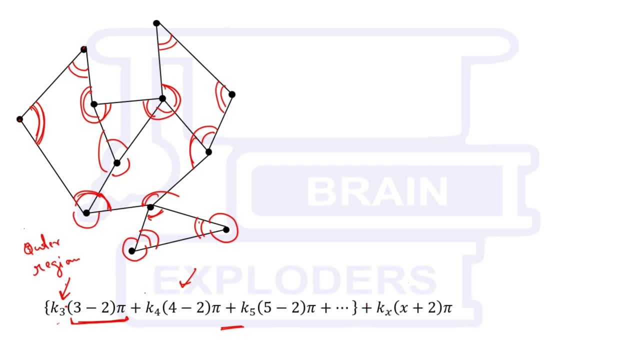 here. So it will add: we are assuming that it has x number of sides. the outer region, or infinite region, has x number of sides. So in this case we are going to add this x plus 2 times pi here. So 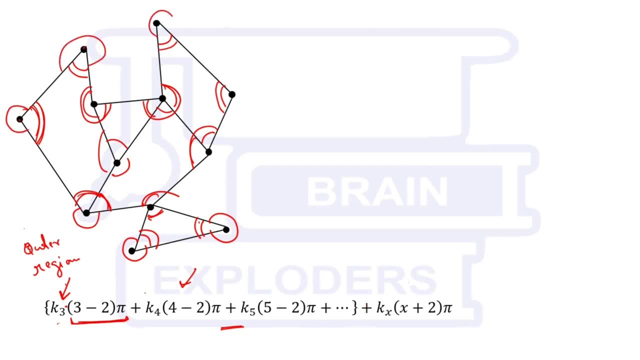 in that case we will add this: these outer regions also, these outer angles, also with this term. So it is going to equal to x minus 2 times pi plus t, What t represents? T represents the sum of angles all around the vertices And this total angle is represented by t. So it is all.